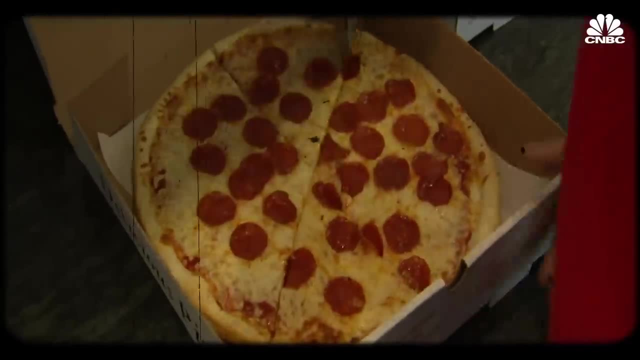 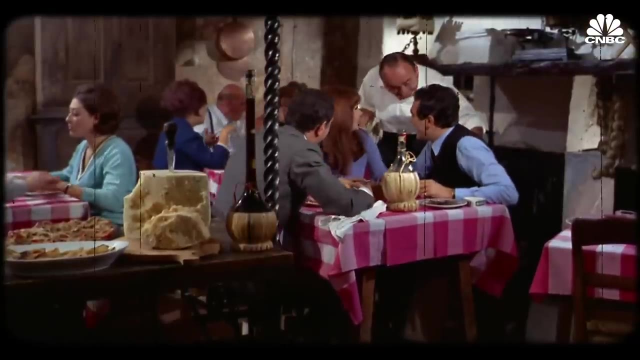 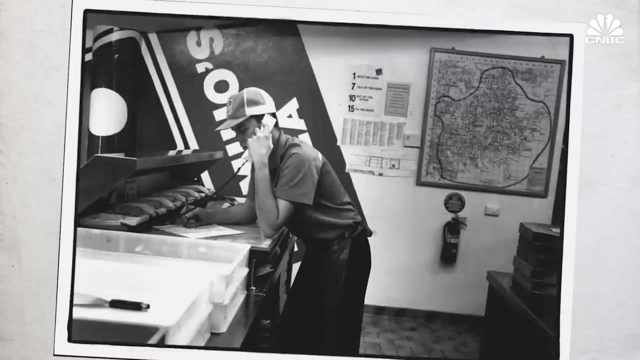 Pizza was once not the American favorite. it is today. Instead. it was a distinctly Italian specialty found in the mostly Italian sections of cities around the country, But in the middle of the 20th century pizza went mainstream Large chains such as Domino's Pizza Hut. 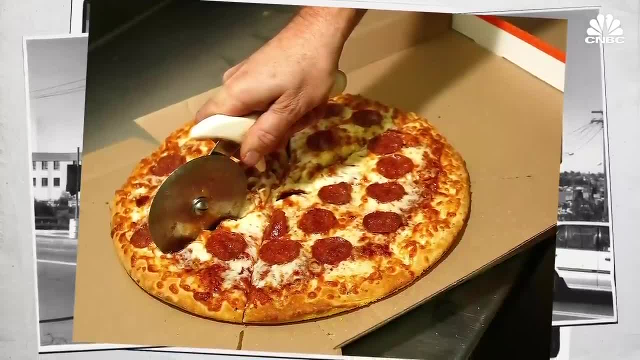 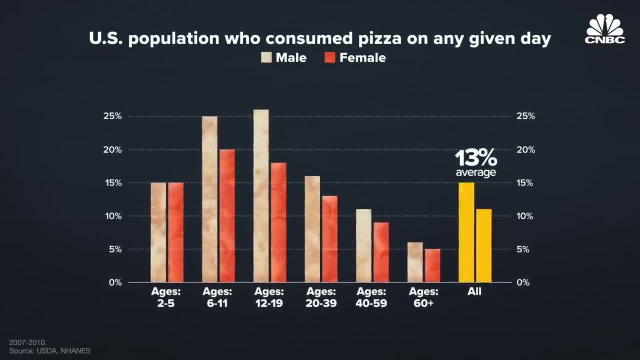 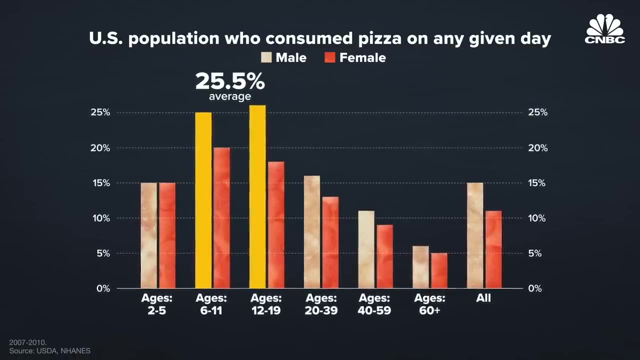 and Little Caesars brought the Neapolitan street food to the masses, and pizza's reach has been growing ever since. A study in 2014 from the USDA found that one in eight Americans aged two years or older and more than 25 percent of all males between the ages of. 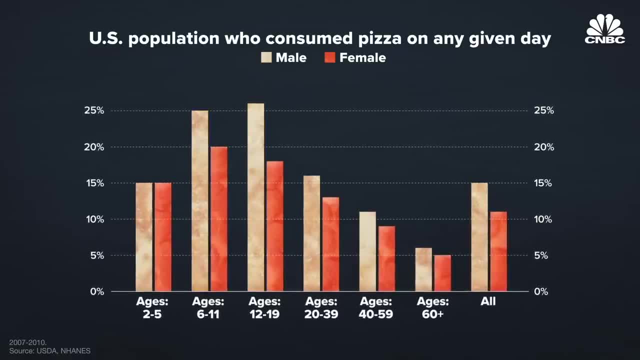 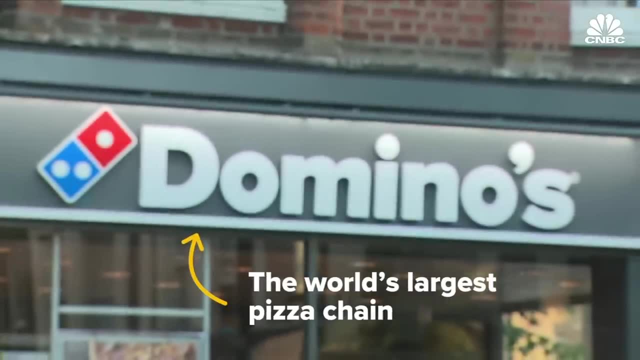 six and 19 ate a slice or more on any given day. The US pizza market was worth more than $45 billion in 2019.. Domino's, the world's largest pizza chain, built its business on perfecting the art of rapidly making and delivering pizza to households around the country. 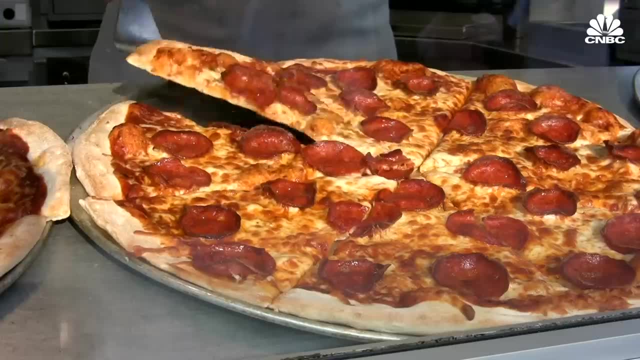 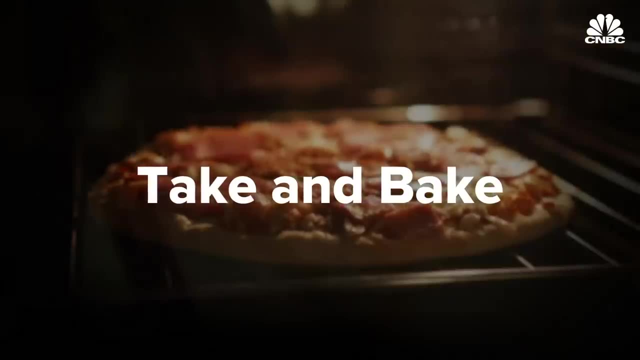 As it has grown more popular. the pizza market has segmented from cheap slices all the way up to gourmet pies. There are sit-down restaurants, carry-out delivery, take-and-bake and pizzas at the grocery store, fresh and frozen. What's happened if you look at the whole pizza category? 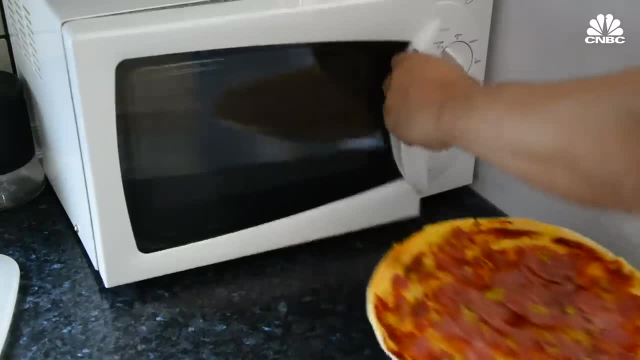 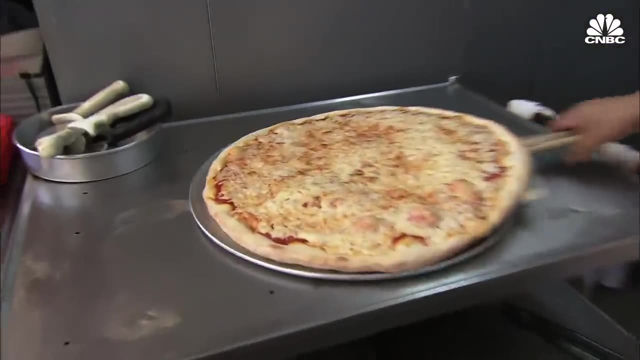 and the cheese piece. you still have that value pizza that you can get for $2 at the grocery all the way up to $20 plus at restaurants, and the continued innovation taking place with brick oven pizzas. Now you know they're selling $5,000 pizza ovens that people are putting in their 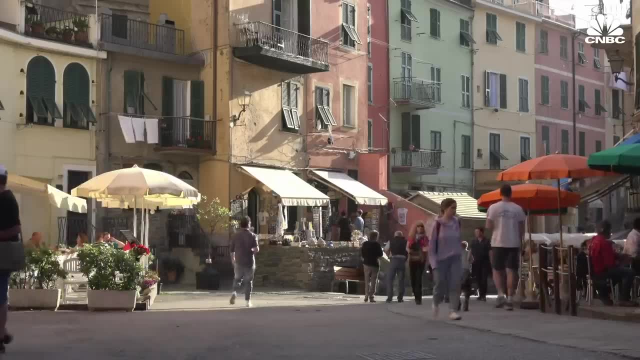 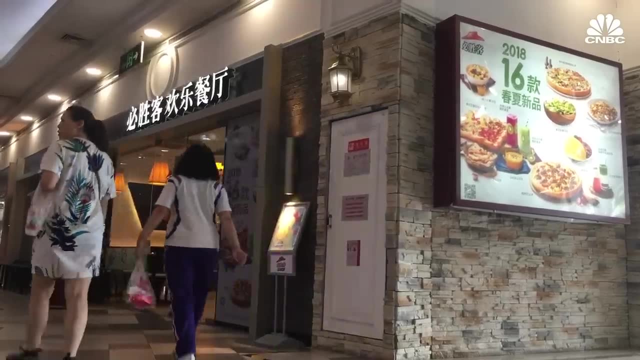 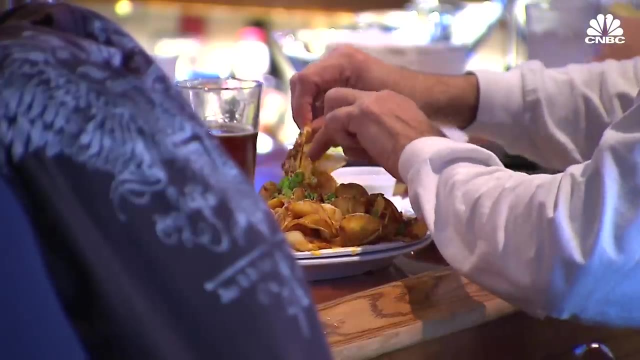 backyard. While pizza is originally Italian, American companies have successfully exported their own version to other countries around the world, even those where cheese is traditionally rarely eaten, such as China. But other varieties of cheese have also benefited from the decades-long growth of food service in the US. The increasing popularity of cuisines such as Mexican and Southwestern-style food, have boosted the popularity of classic American-style cheese varieties such as cheddar and Jack. We partner with Taco Bell. we started working with them in 2012.. They used to view cheese as a garnish, like lettuce and tomatoes. 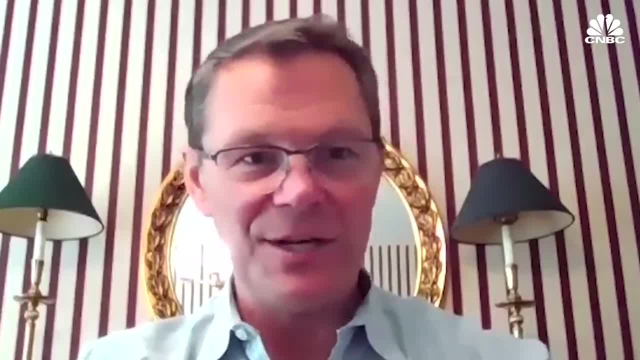 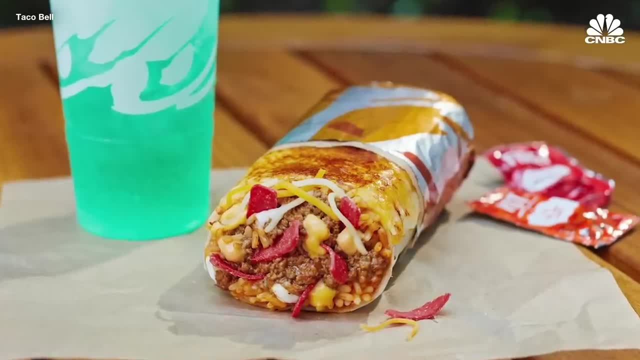 and we started showing them all these new innovative properties that cheese can do. You know, now they stuff the shell with cheese. You know we just launched with them a grilled cheese burrito where actually, you know, it's got cheese sauce on the inside and a melting cheese. 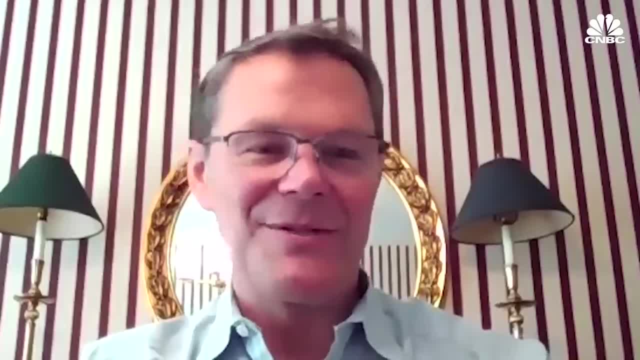 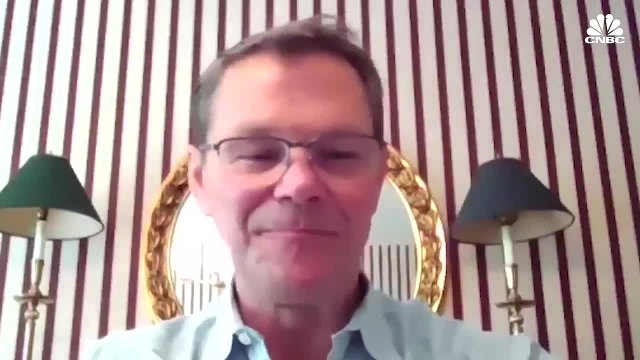 on top. Their consumers love the transformative properties, and so that's just a really fun thing that you see why it's so important to the consumers- because they can use it in so many different ways, The way mozzarella has been able to piggyback on pizza to achieve its popularity. 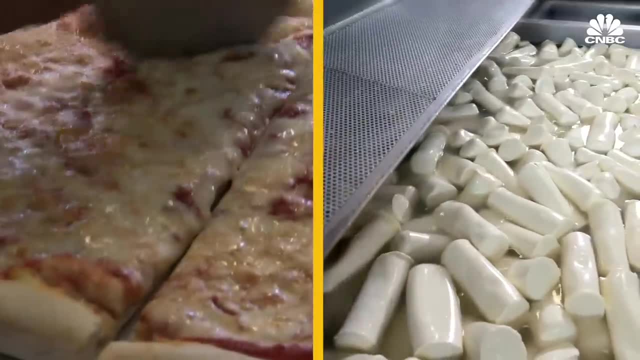 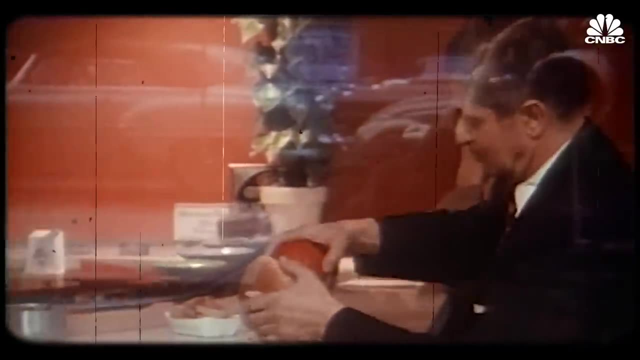 says a lot about how the fate of one food product is often tied to that of another. In the middle of the 20th century, another cheesy substance rode high in the US, in large part on the popularity of another classic American dish, the fast food hamburger. 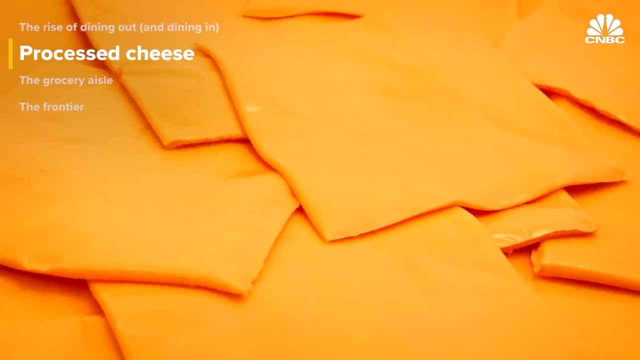 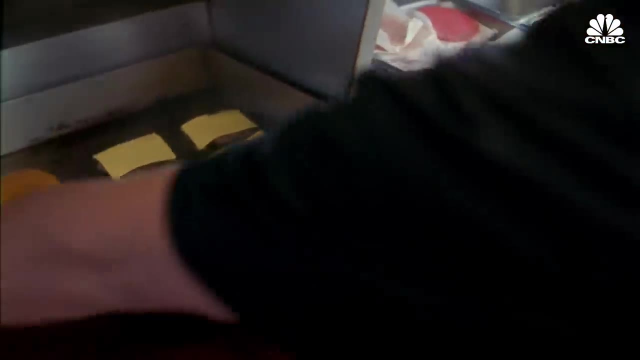 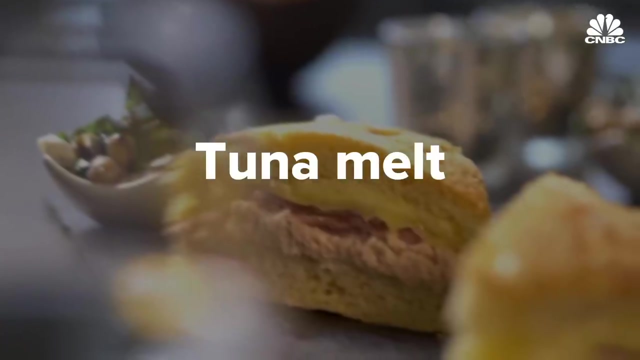 It is hard to talk about the history of cheese in America without talking about, well, American cheese. The yellow orange slices are famed as essential components of classic American diner staples such as cheeseburgers, grilled cheese sandwiches and tuna melts. American cheese is a processed cheese, which means it is made from cheese and some other ingredients. 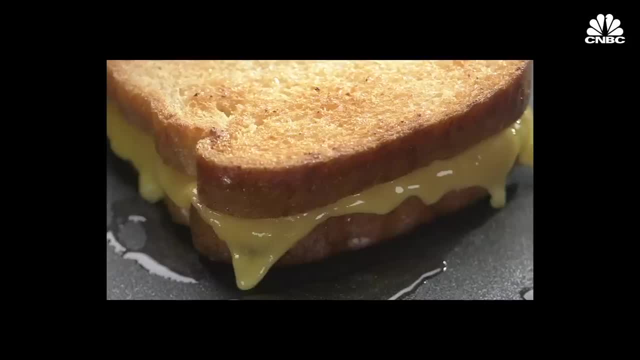 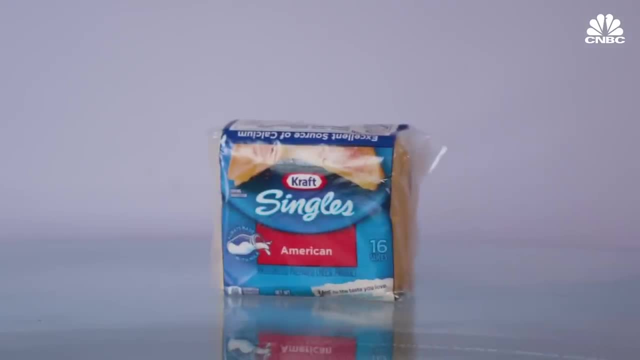 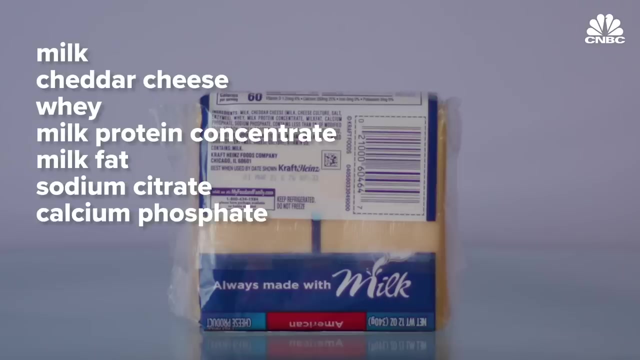 that, among other things, help prolong its shelf life and allow it to be smoothly melted. Perhaps the best known brand of American cheese, Kraft Singles are made of milk, cheddar cheese, whey, milk, protein, concentrate, milk fat, sodium, citrate, calcium, phosphate. 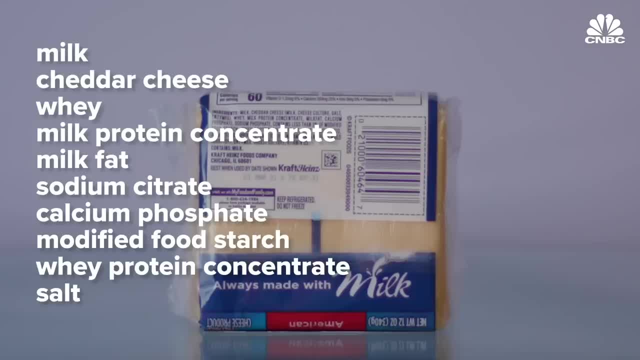 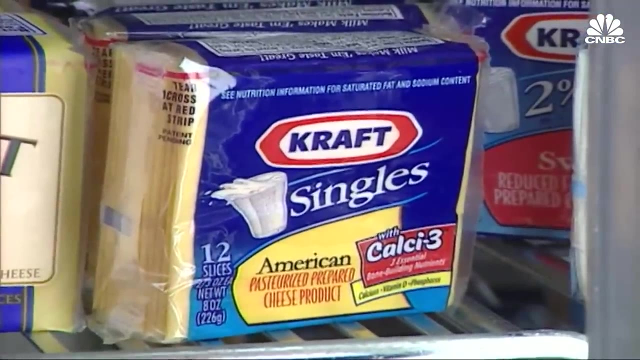 modified food starch, whey, protein concentrate, salt, lactic acid, annatto and paprika extract for color, natamycin, enzymes, cheese culture and vitamin D3.. Apart from slices such as Kraft, singles processed cheese also refers to products such 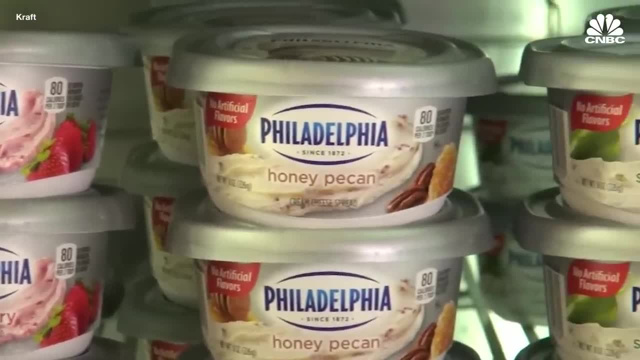 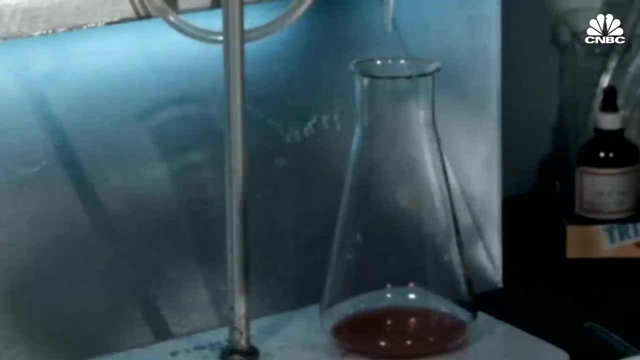 as Velveeta, and a range of spreadable cheeses such as cream cheese, and cheese products such as Easy Cheese and Cheese Whiz. It appears a few different groups of food scientists were working on recipes that would become what we know as American cheese. 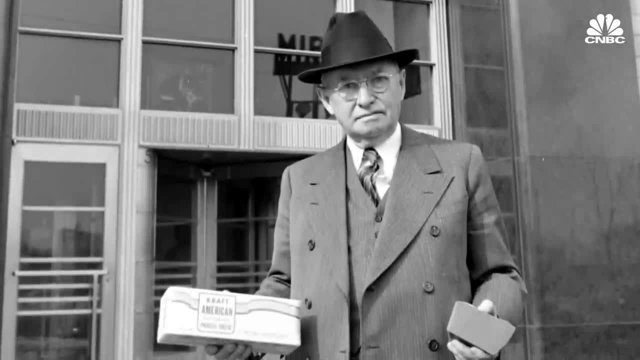 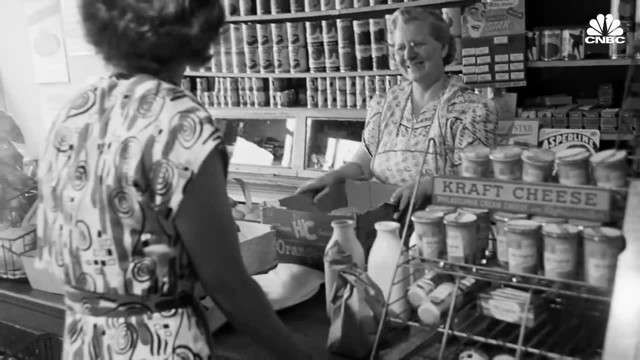 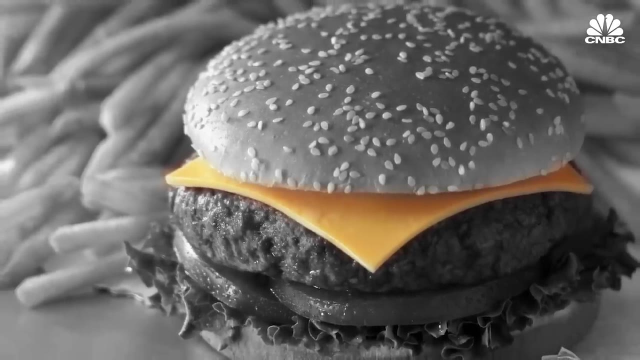 But in 1916, the Canadian-born American businessman, James Lewis Kraft, patented the process for producing the American cheese that would make the Kraft brand name famous. Later, American cheese became a staple ingredient on cheeseburgers served all around America and later around the world by fast-food giants, perhaps most famously McDonald's. 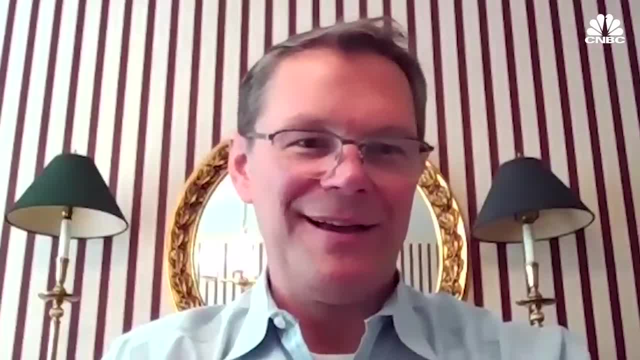 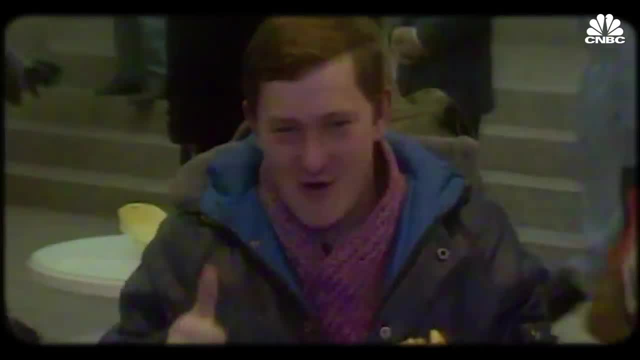 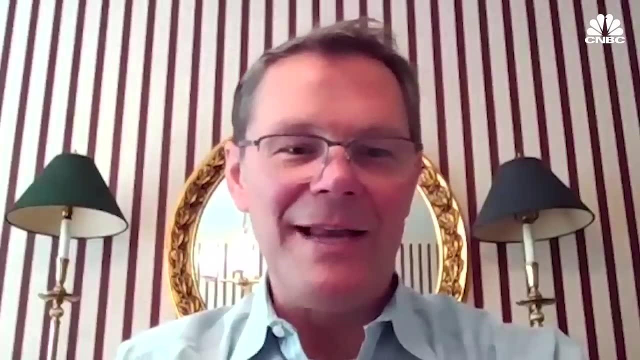 You look at it like it's McDonald's right. The launch of that chain and the launch of the hamburger using American cheese on that kind of just helped install that culture in the world. And I always still tell people the fun fact: if you think about it: 85% of cheeseburgers. 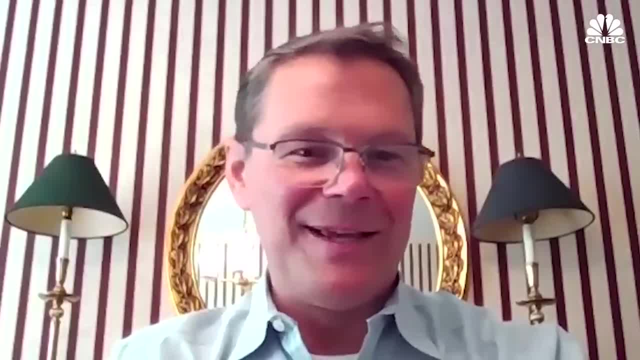 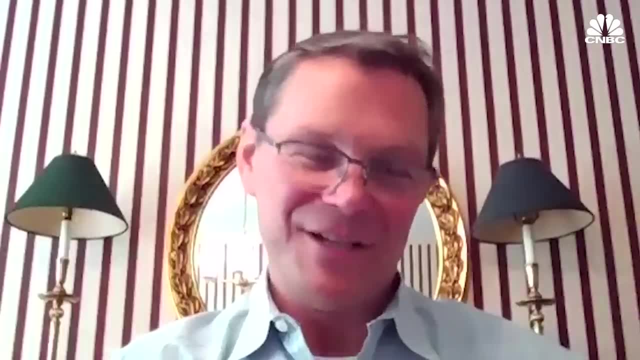 have cheese on it and only about 10% of chicken sandwiches have cheese. but I would much rather have the taste of beef versus the taste of chicken. They're kind of side by side. they're kind of chickens: blander, yet they put more cheese. 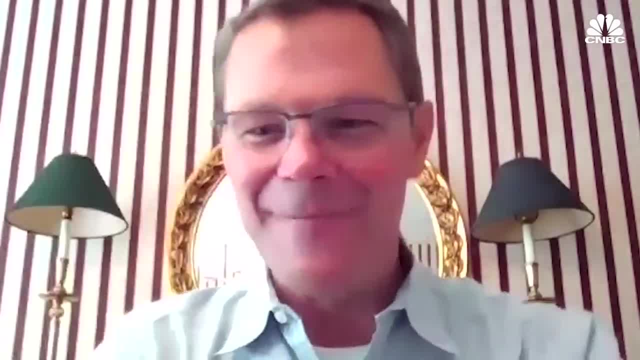 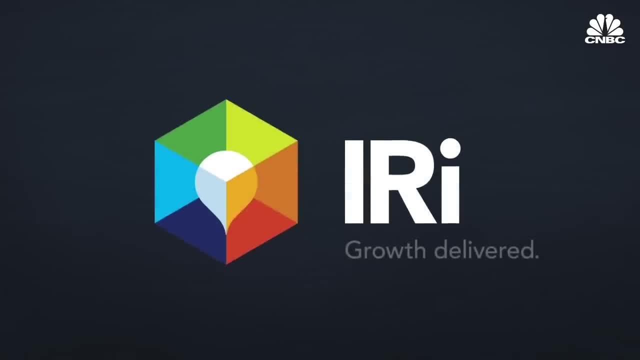 on beef and chicken, So chicken's an opportunity when you think about that. However, processed cheeses have declined in popularity over the last decade or so. For example, industry research group IRI told CNBC that processed cheeses such as slices and spreads. 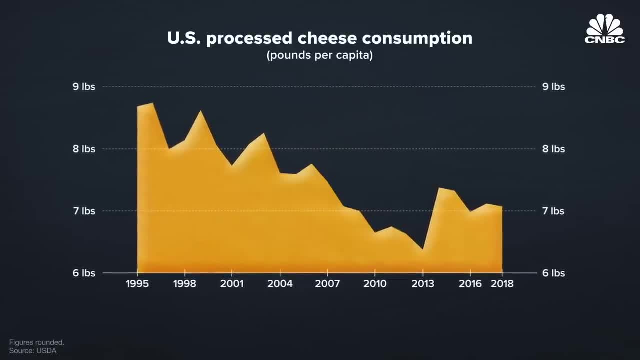 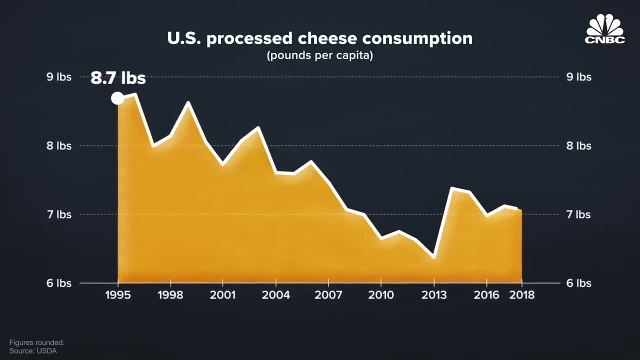 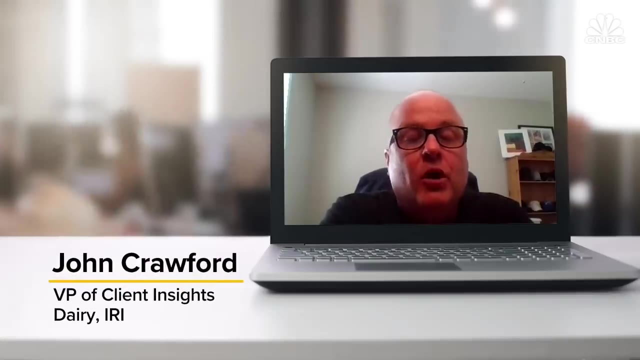 sold in the cheese section of the grocery store dairy aisle have seen sales decline nearly 18% since 1995, from 8.7 pounds per person that year to 7.07 pounds in 2018.. So there's a couple of categories within dairy that have been struggling over the past. 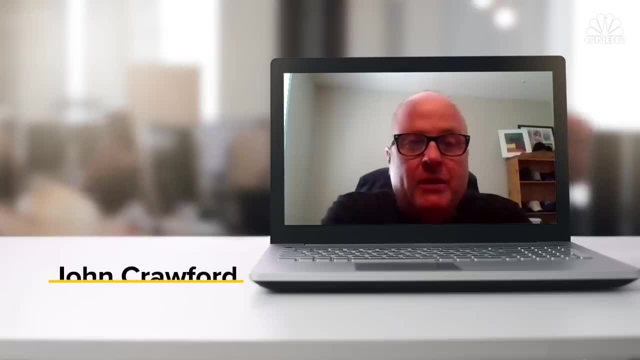 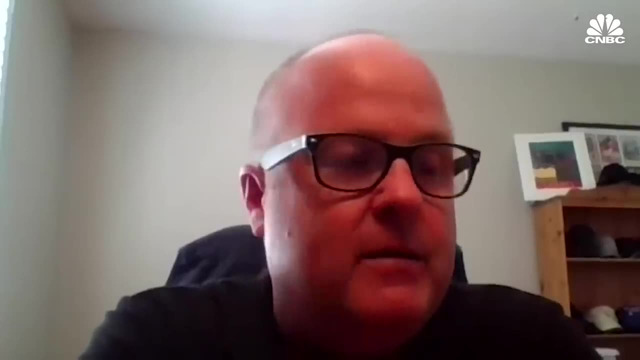 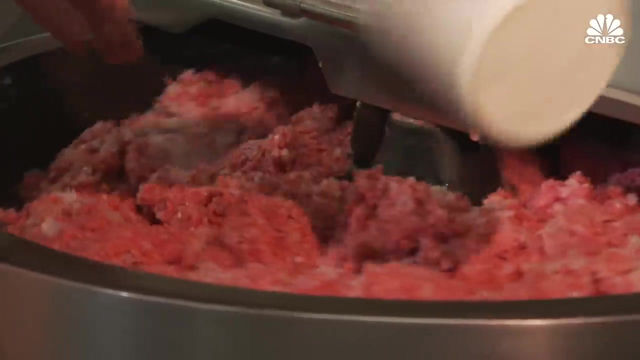 few years, one being processed cheese and one being margarine, And so you think about how consumers have moved away from processed foods. processed cheese, and cheese And and margarine have really struggled over the last five years. Processed cheeses, like processed foods in general, have their critics who say these: 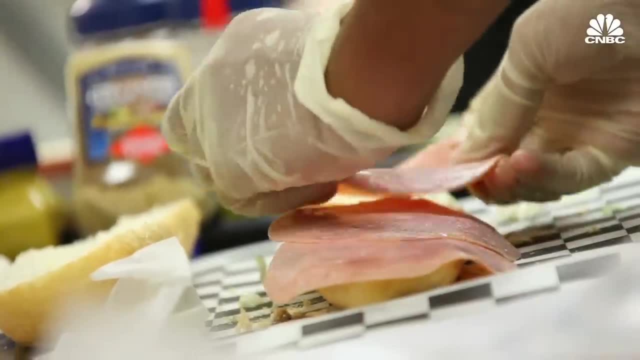 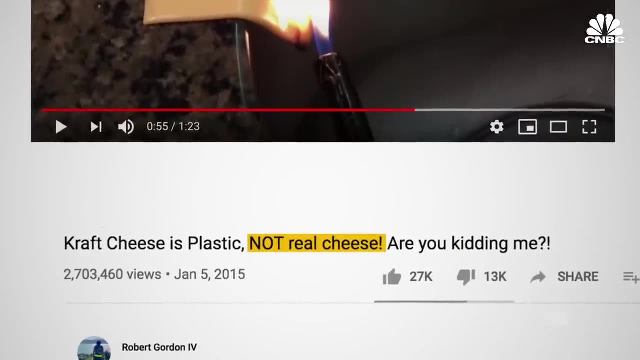 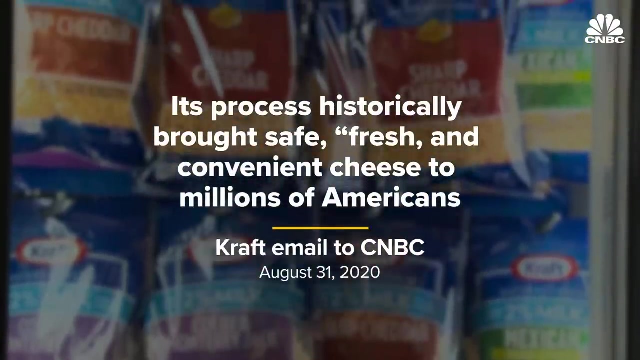 long-loved goods are unhealthy examples of America's misapplication of industrial manufacturing methods to food. It is not even cheese, say some haters In a comment to CNBC. Kraft said its process historically brought safe, fresh and convenient cheese to millions of Americans at a time when that wasn't the norm. 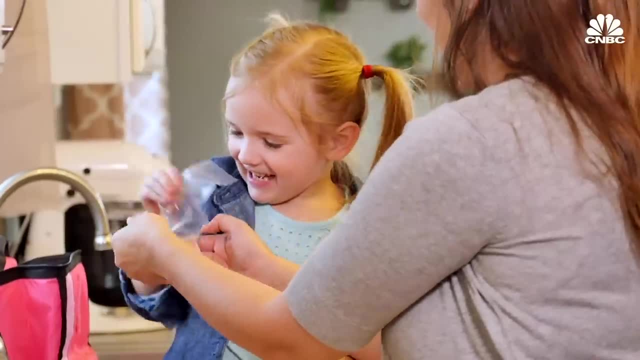 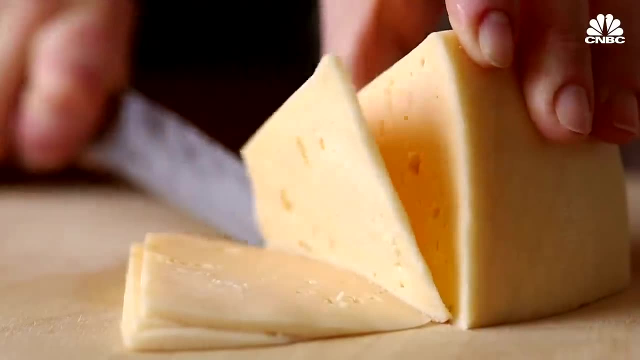 And that's not true. That's not true. That's not the norm. American cheese continues to be popular in over 60% of households. Kraft also said it makes over 30 flavors of natural cheese in a variety of cuts. Some industry analysts think the decline has to do with these consumer concerns and with 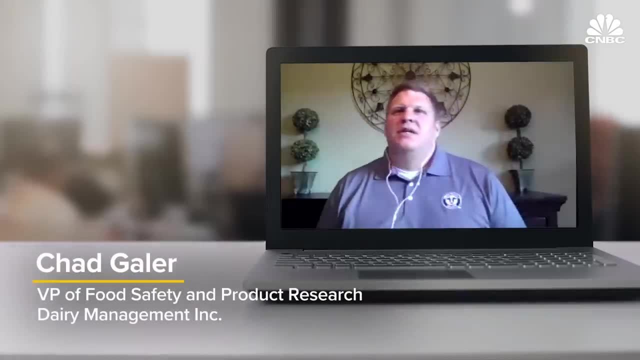 the way processed foods are labeled. Processed cheese has you know, I think it suffers from having a nomenclature that you know from the Code of Federal Regulations. its name is processed cheese and that has to be on the package. 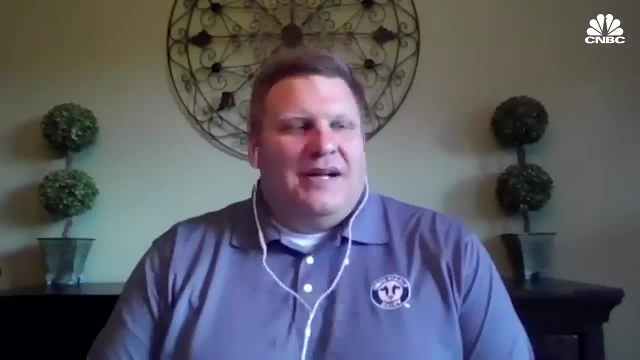 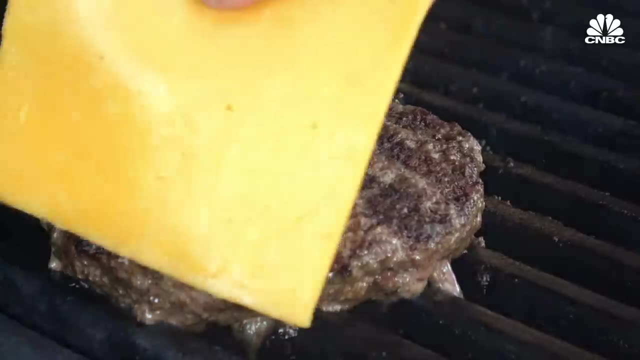 You know legally. And what does processed mean? A lot of them are, you know, all dairy. It just allows it to have a longer shelf life and the science behind it allows it to melt just beautifully, and that's why it's so great on a burger, because it's just got that. 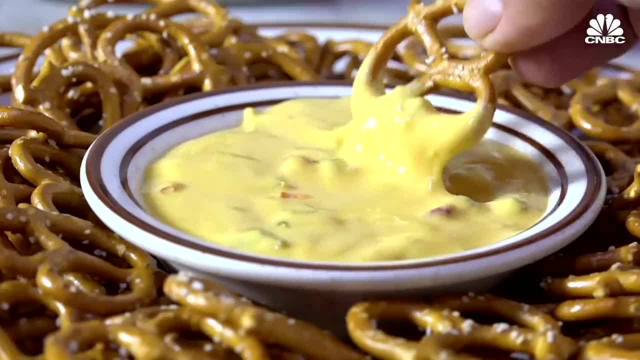 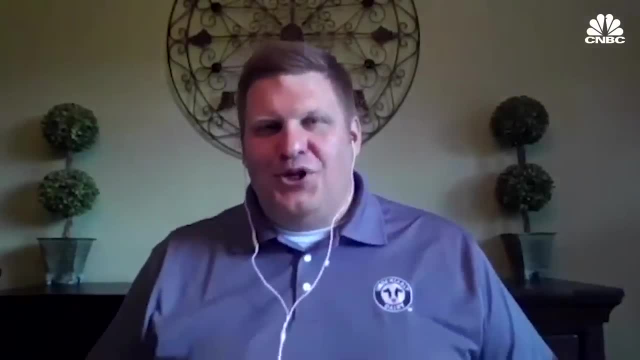 perfect melt. You know, if I want to make a cheese dip, there's not much better than a processed cheese to put that together, because if it's smooth melt it's not going to oil off. That's the properties it owns and it should have. 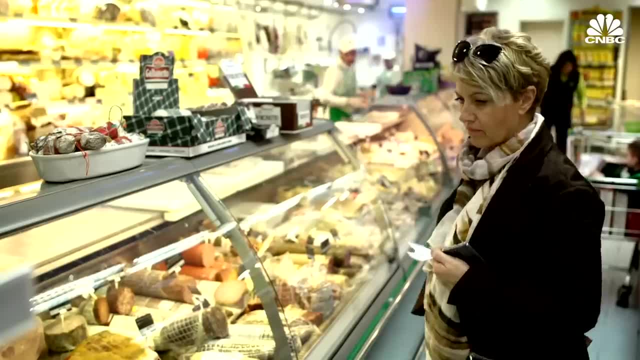 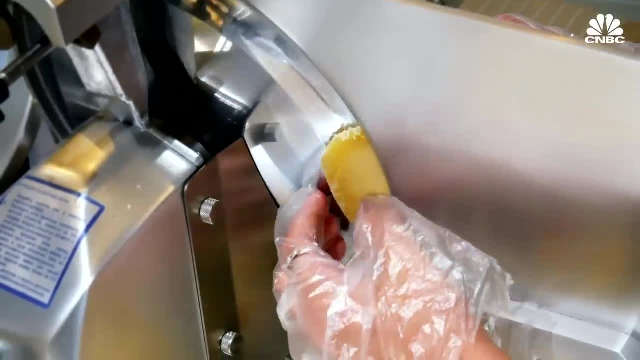 Interestingly, while grocery sales of processed cheese are down, customers ordering cheese or sandwiches with cheese at the deli counter, whether in a grocery store or elsewhere, seem to be opting for American cheese, the processed kind, at about the same rates they have in. 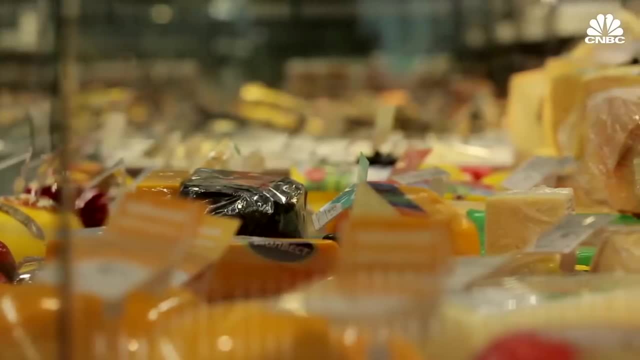 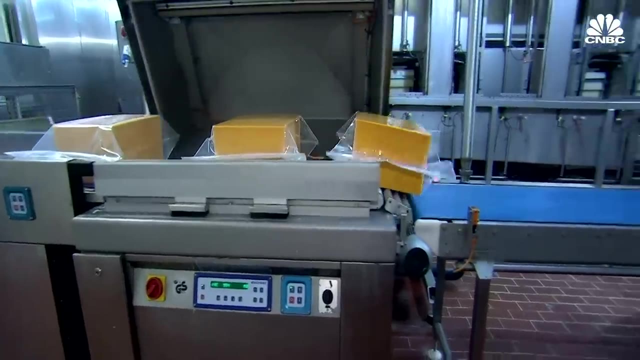 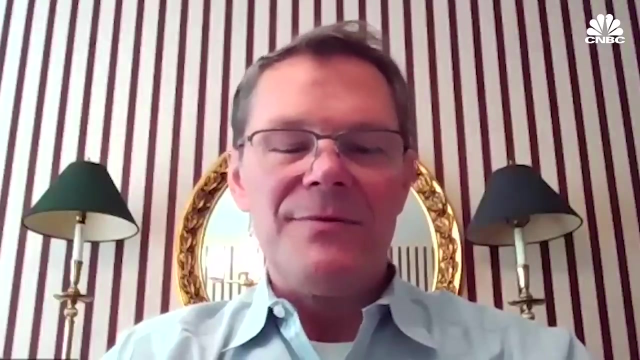 the past. Another reason why processed cheese might be falling out of favor is that technology for packaging natural cheese has improved tremendously, undercutting the need for preservatives When you're shifting forward to the category. Basically, what happened was it was the introduction of all the new flavor cheese and also product. 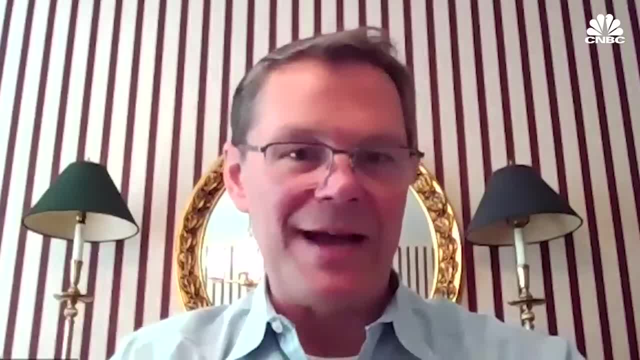 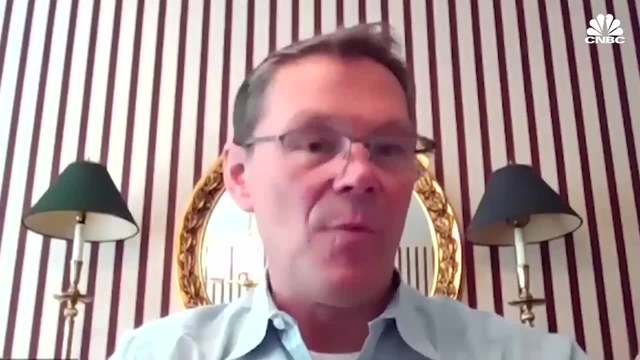 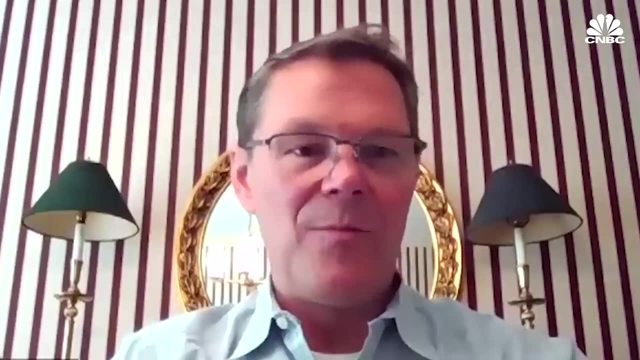 I'll call it the packaging systems: higher quality package of preserving systems to enable natural cheese to be launched and stay without molding. You know, if you look at like the sliced sandwich cheeses today, you know you definitely need to. you know they call them multi-vac systems to be able to preserve, shut and seal you. 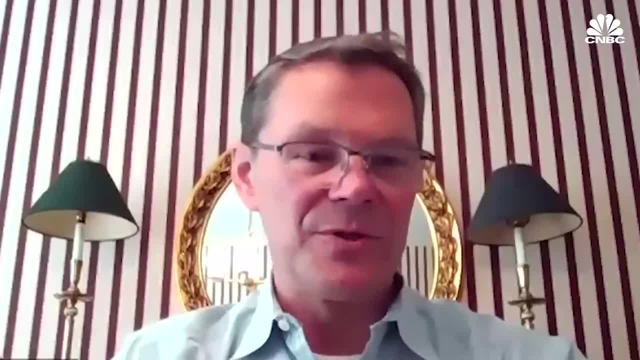 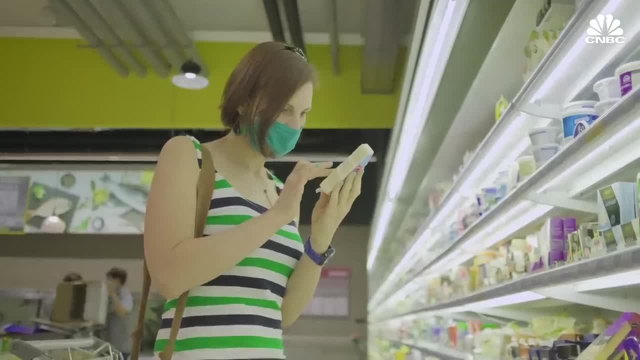 know, You know, with less preservative, right, because they don't. they have zero preservatives like the natural cheese or the processed cheese has. It is notable, however, that processed cheese has seen a bit of a resurgence of interest amid the coronavirus pandemic. 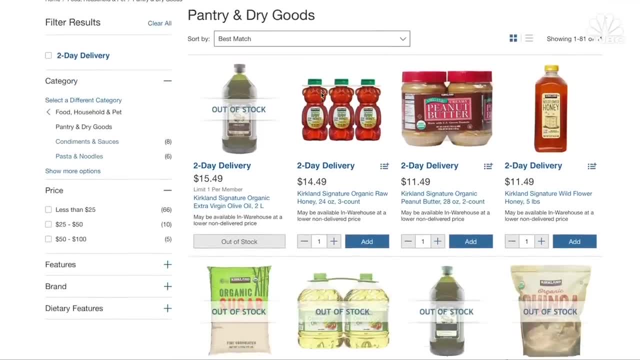 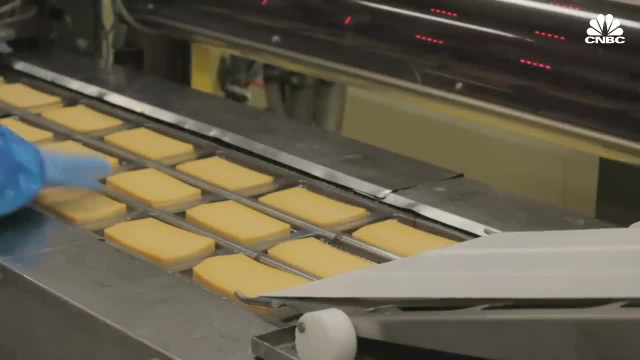 With more people cooking at home, stocking their pantries and perhaps eager for nostalgic comfort foods, the fact that processed cheese is processed might actually now be a selling point. But consumers, now with with faced with you know, wanting to have something you know. stuff, products that had a longer shelf life, that maybe were canned. you know they were shopping in different, different sections of the store that maybe they hadn't shopped in before. Kraft macaroni and cheese, I think, had a huge- you know, a huge- uptick in terms of 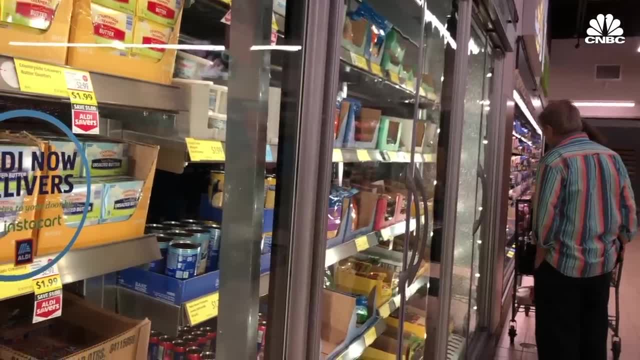 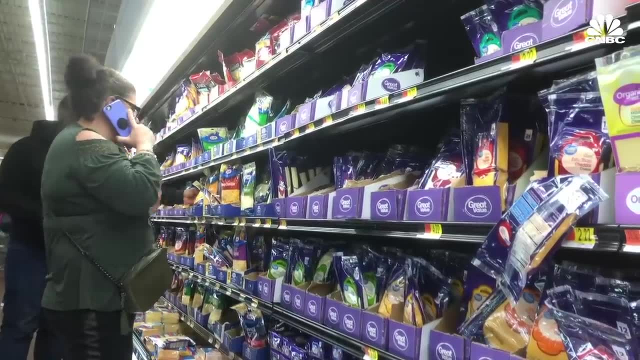 in terms of the volume that it sold during COVID. But what we what we saw was we saw processed cheese and margarine all of a sudden see some pretty good growth, which we hadn't seen again for like the last four or five years. 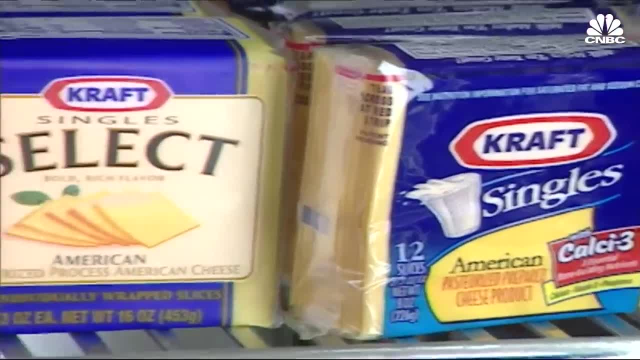 Kraft told CNBC it has seen double-digit growth in its singles products- And it's not just a single product, It's a double-digit product. It's a double-digit product, It's a single product in 2020- and pointed out that Internet searches for grilled cheese. 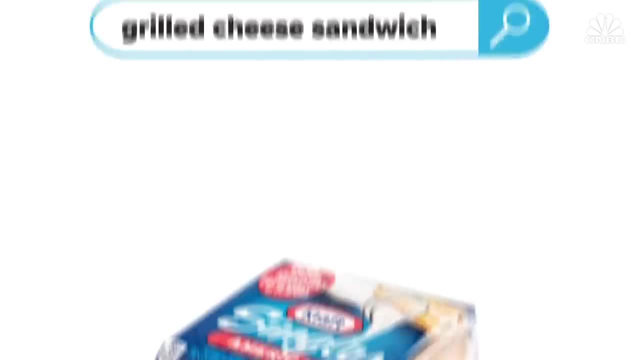 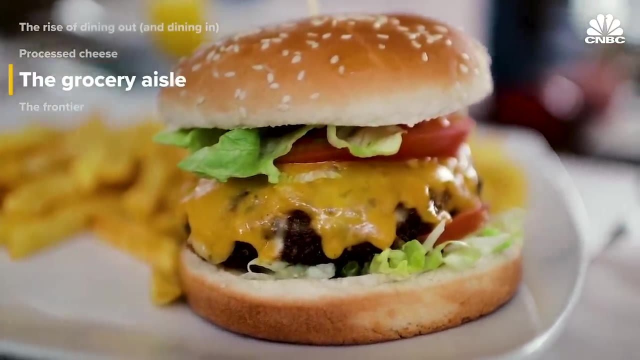 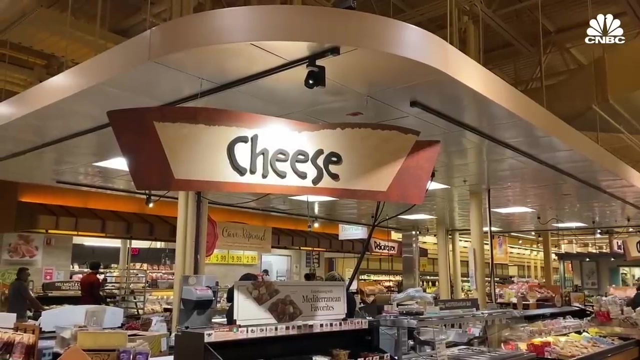 sandwiches, which frequently feature Kraft singles, are up 30 percent, While restaurants are largely behind the rise of cheese eating in America. what consumers are buying at grocery stores also shows how the cheese market has changed. Stores are stocking ever greater varieties of cheese in an array of forms to make it. 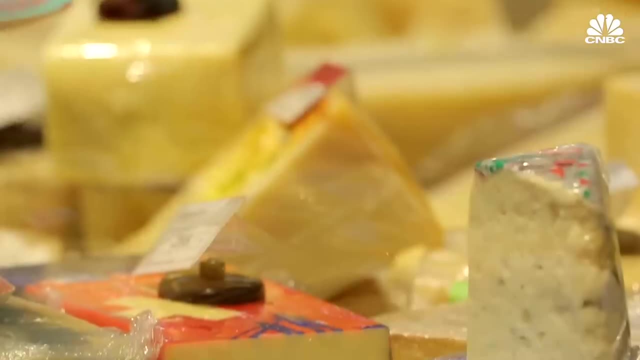 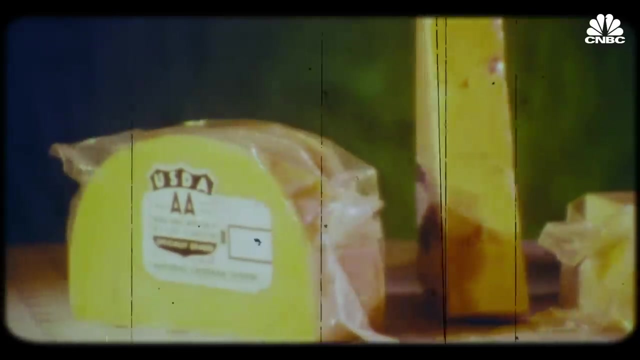 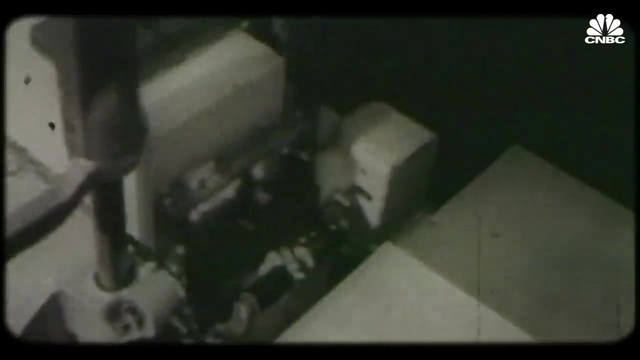 easier for customers to incorporate cheese into their diets. The aforementioned changes- Changes in packaging, have had a huge impact, and not just on processed cheese. Historically, grocery store cheese was sold mostly in blocks. Over the last few decades, companies have found ways to package cheese for convenience. 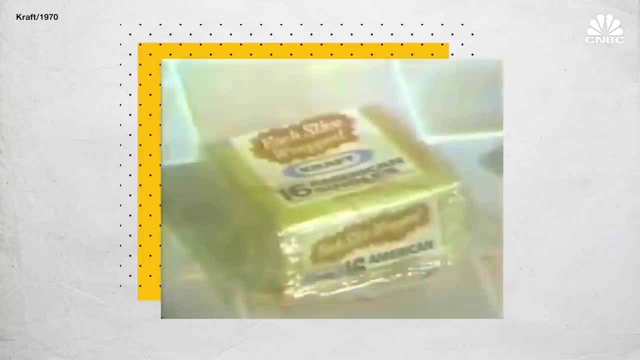 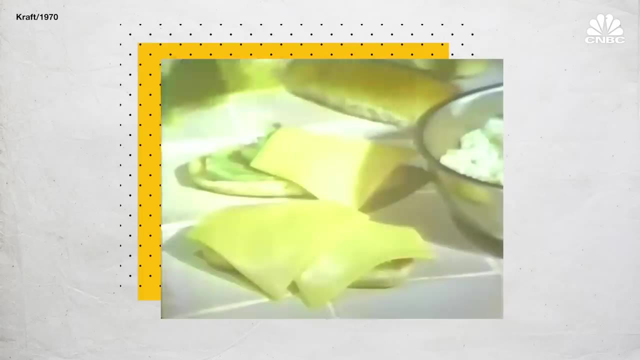 and to market new categories of products for customers. Kraft American singles. These pasteurized processed cheese food slices can make your basic tuna salad sandwich pretty special. They're individually wrapped so they're easy to open. Sometimes all a company has to do to induce customers to buy a cheese sandwich is to 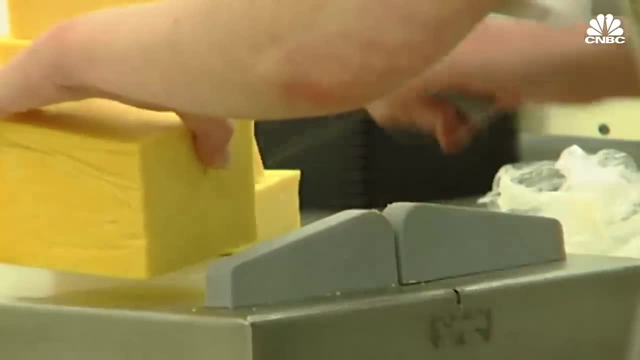 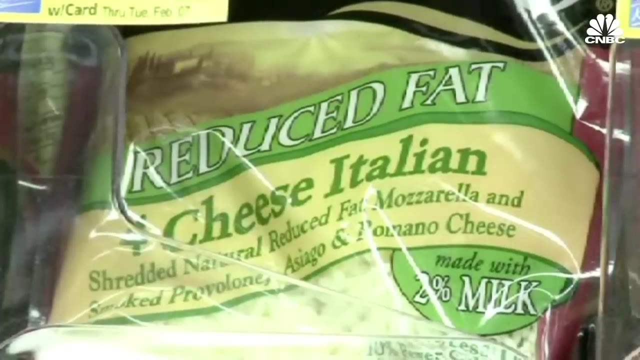 go to Kraft, Kraft American singles. The first thing you need to do for customers to buy cheese is cut it for them. For example, those bags of shredded cheese you see everywhere. They came about in the 1990s when the process for easily shredding and packaging large amounts 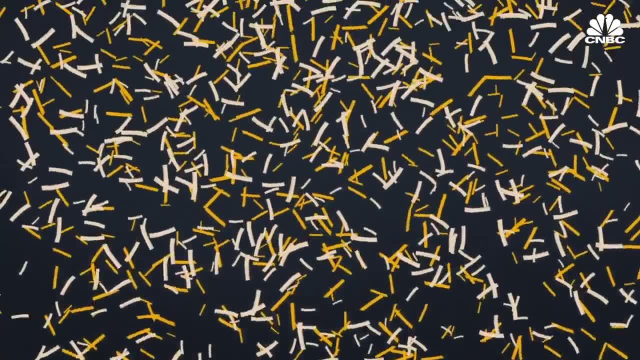 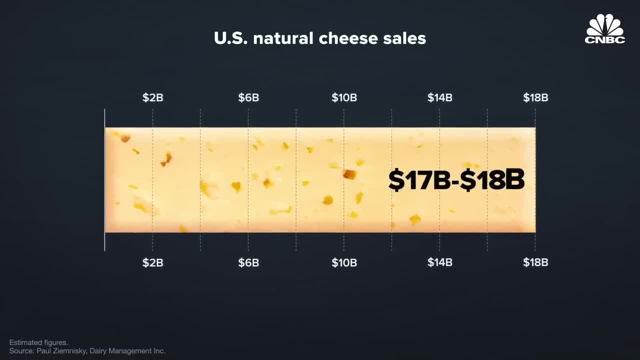 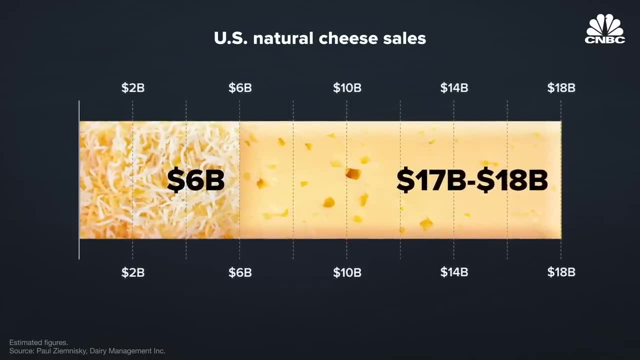 of cheese was developed. Now shredded cheese is the biggest seller of natural cheese varieties. The entire natural cheese category is worth around $17 to $18 billion and shredded cheese alone is about $6 billion of that. Customers like the convenience. One of the things we looked at is, once you put a shredded cheese in the household, they 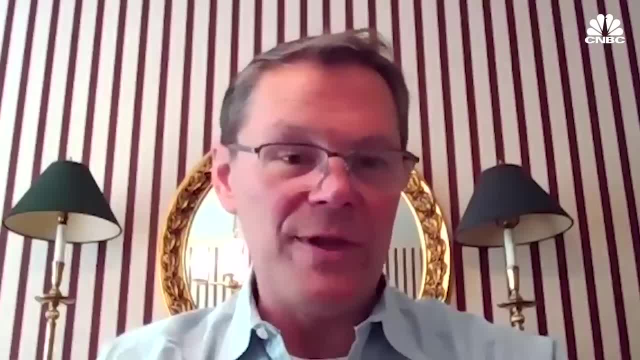 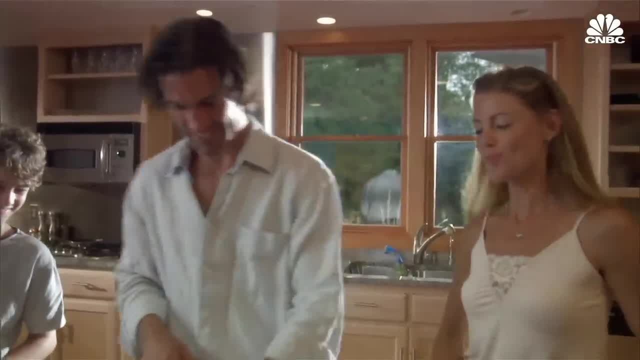 just use it so many different ways. I think about a quarter of the use of it was just people snacking out of it. If you're making an omelet, people still snack. If you're making a quesadilla, they were still snacking before they even made the quesadilla. 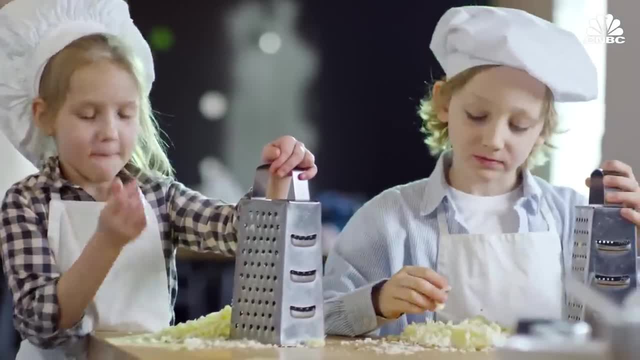 It just became a snacking device and that actually led to different snacking forms being introduced. when you go in homes and do the ethnography with the products, That's where you see a lot of people snacking. That's where you see a lot of people snacking. 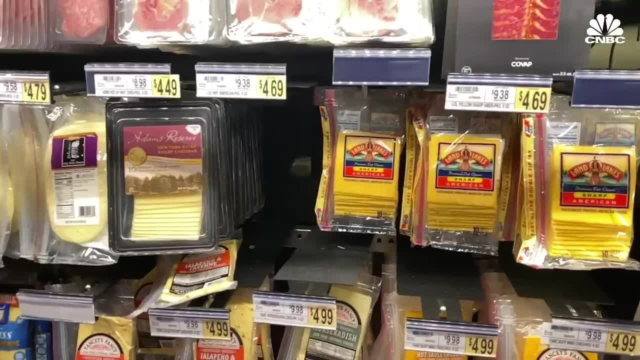 That's where you see a lot of people snacking. That's where you see a lot of innovation take place. Well, how are you using this? There is also pre-sliced natural cheese, which is sold in what are called shingle packs.